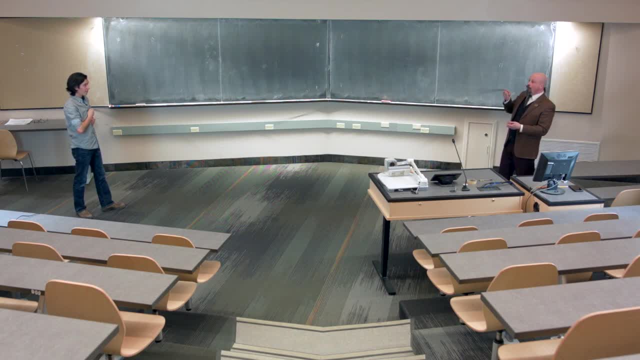 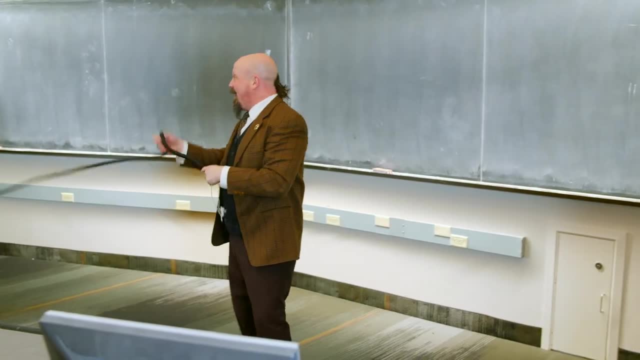 a half wavelength, Increasing it again. we can put in another half wavelength interval, creating one full wavelength or two halves. Now this is a mechanical wave, It's a wave trapped inside of an actual object, But something else that behaves like a wave is something. 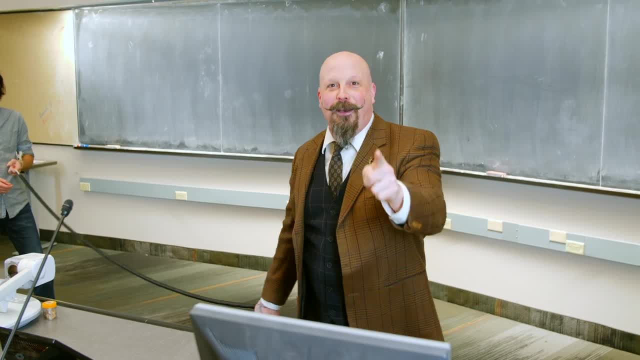 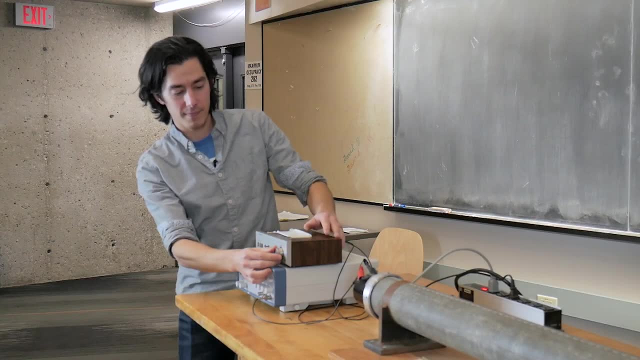 that we call sound waves, Sound. So sound is also a wave, right Yeah. And so you can actually generate sound with a speaker system like we have over here, In the same way that we established a standing wave on the spring, that mechanical wave. 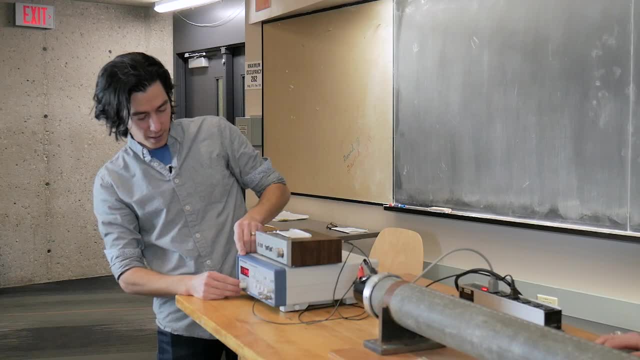 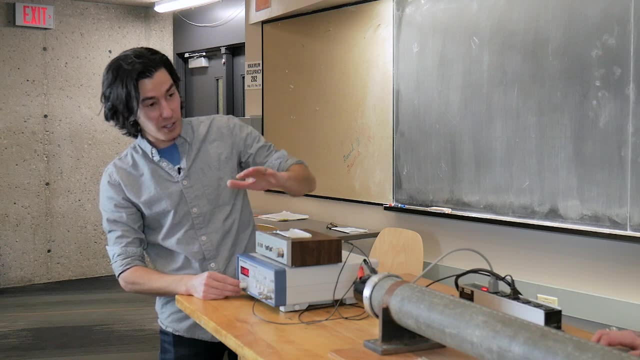 we can do the same thing with sound. Sure, if we just change the wavelength of the frequency, you'll hear it get louder just when we get to resonance. So you can hear as I change the wavelength up and down, And that's not increasing volume over there. 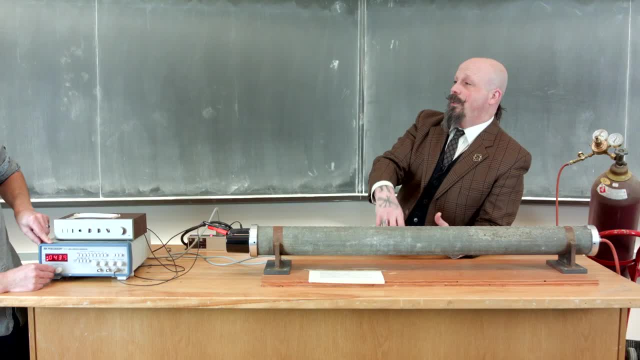 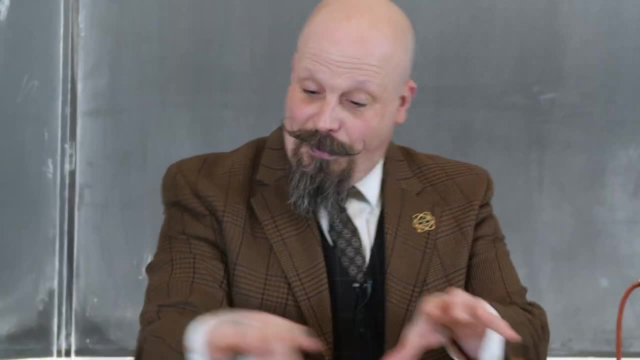 that's just by changing the frequency. So the frequency comes up to some resonance level and then as you go past it it actually gets quieter again because you've put them in in non-half wavelength intervals. Now that's the sound waves inside of here And you can hear it. 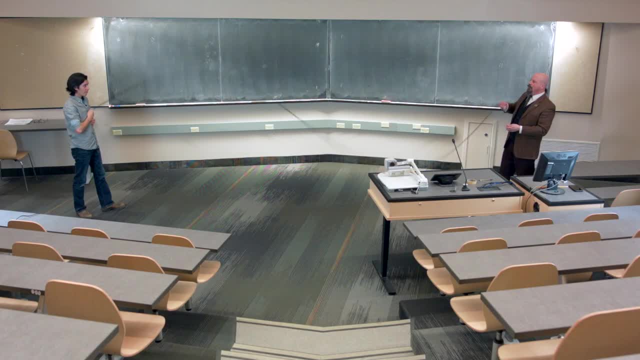 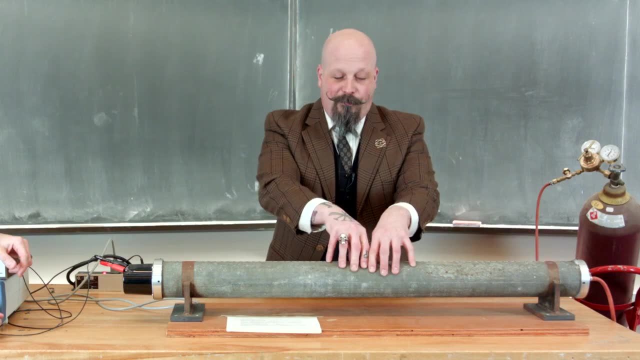 but you can't actually see it. It's the same thing as the mechanical wave that we just saw, But let's take a look at it. What does it look like? So what we've done here is we've taken this tube and we've filled it full of methane gas. Now we've 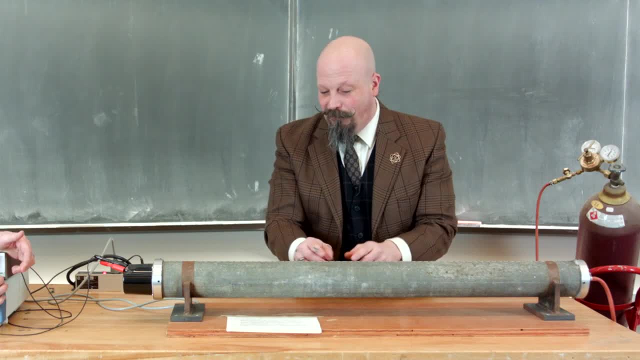 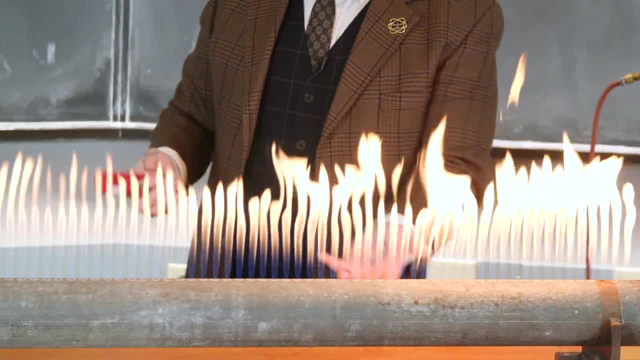 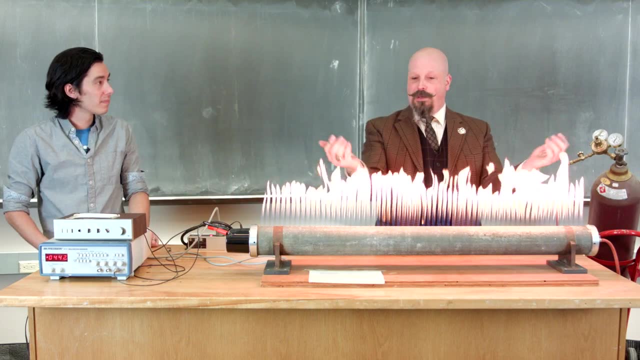 three quarters of an inch, And if there's gas coming out, it's going to be three quarters of an inch- Then you can light it on fire. This flame indicates that there's actual gas inside of this tube, right And right now there's no sound, So this gas just coming out completely on its own. 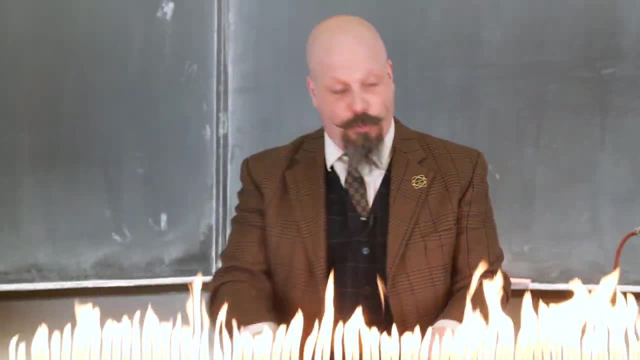 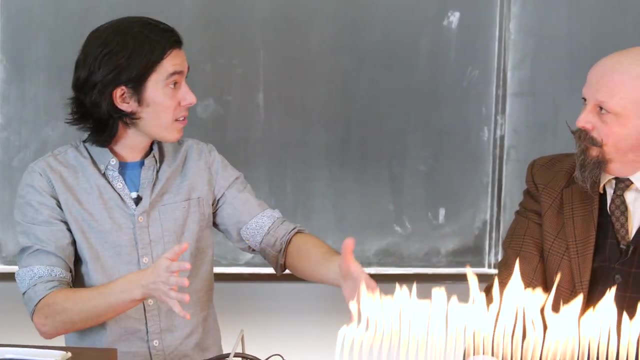 we've got an even level of distribution. I'd say the pressure is probably the same throughout this entire tube, And what we're going to do is we're going to send a standing wave through here and that's going to alter the pressure at different points We're going to get resonance. 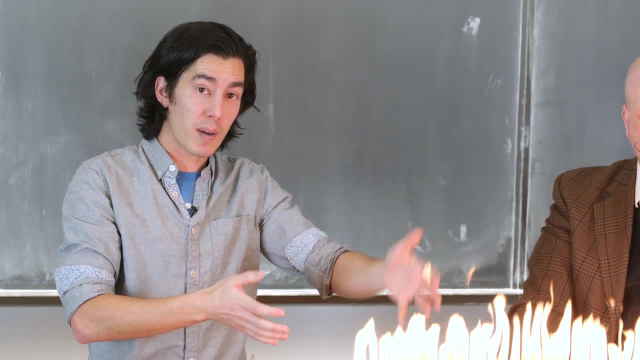 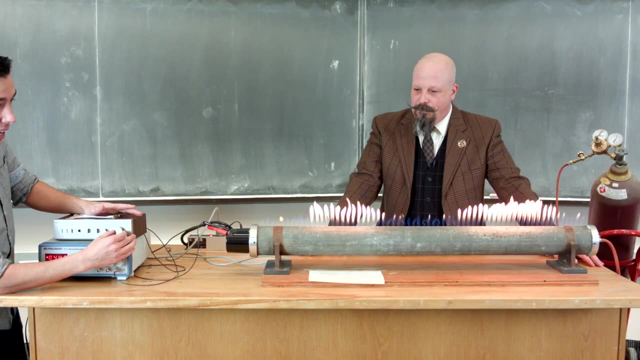 and so there are going to be parts where the pressure causes a large flame to come out and other regions where the pressure inhibits the flame. Here I'm just going to turn the sound up a little bit And you can see right in the middle we have a low amplitude of the flame. 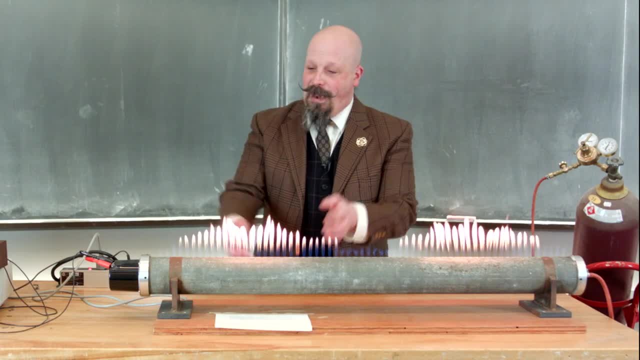 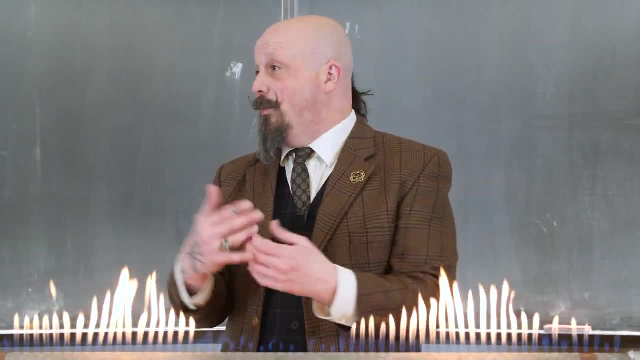 And it's in half wavelength intervals, right, We have a half wavelength here and a half wavelength here, And so you've got a whole wave. that's in here, Constructive and destructive interference taking place just from the sound that's being pumped into this tube full of gas. 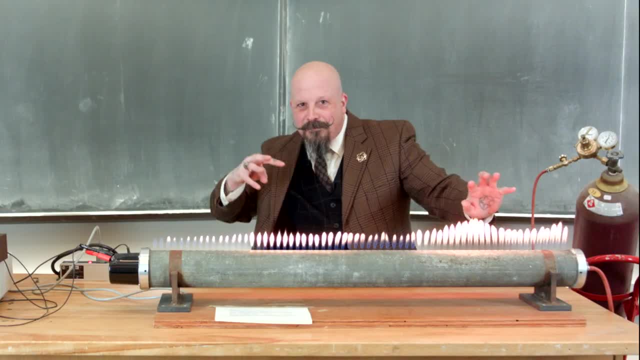 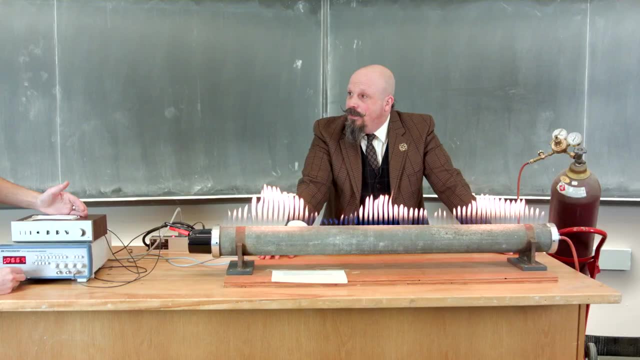 If I tune this up a little bit further, you'll be able to hear me get resonance again when the volume goes down. There we go. I think that's a very, very low-. So this is three half wavelength intervals, right? Just the same way as we had in the spring. 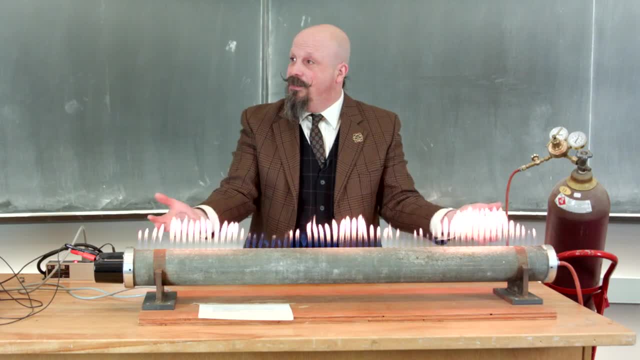 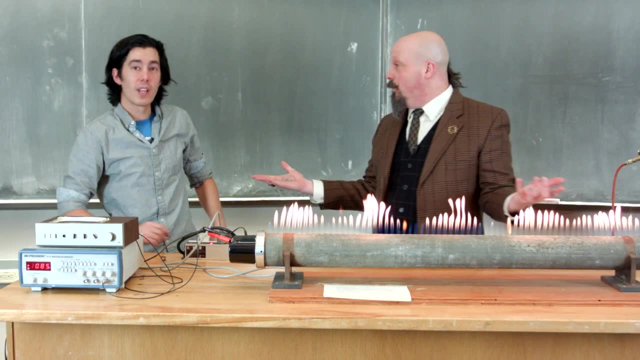 the mechanical wave. now we've recreated that with sound waves inside of a tube just oscillating the pressure from high and low versions of pressure. This is a one-dimensional representation, just exactly the same as that spring that we saw before 1D Straight line comes here, bounces, pops right back and comes right back at it. 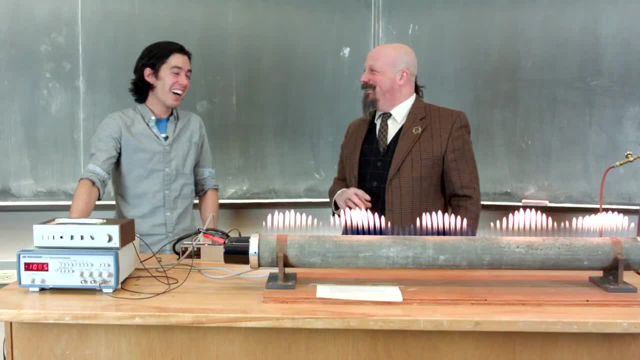 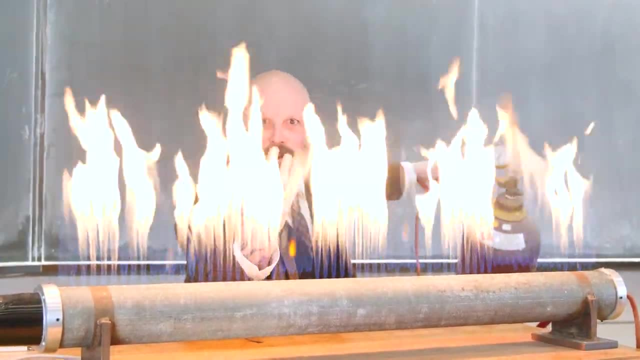 You can actually take this and adapt it to a 2D surface. Okay, let's check it out. All right, You know what will fix this? More fire Segway through the fire Segway through the flames and Before. we were looking at a one-dimensional example. 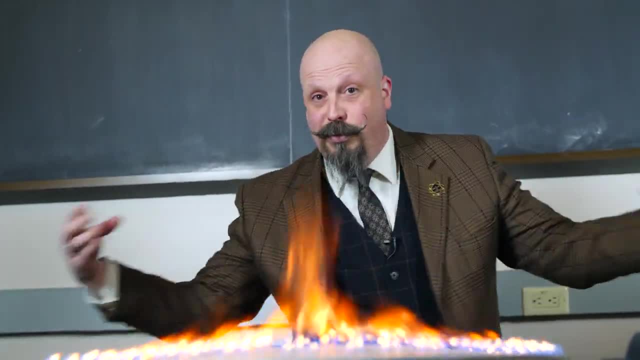 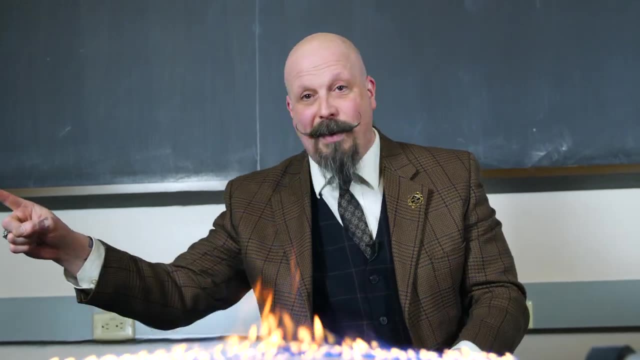 where we watched a wave travel along a spring. we watched a wave travel through a tube. but we can actually also look at a more complex example in two dimensions. Here we've got a flame drum Now instead of just a wave going from one end to the other. 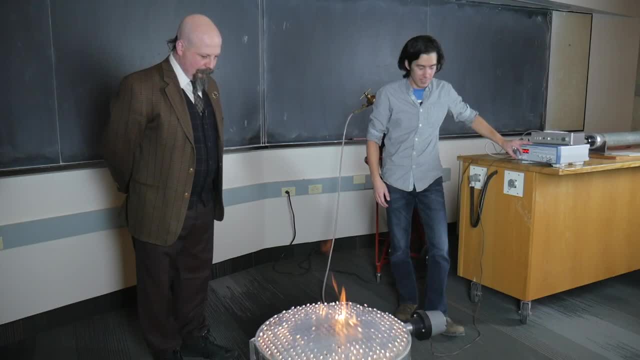 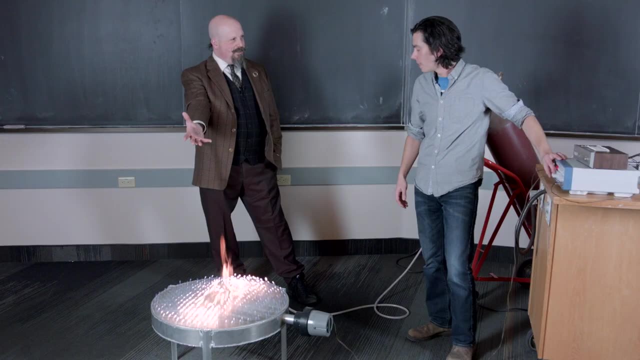 it's free to exist in this 2D environment, And so you get the same thing right: Resonance: you can hear the resonance audibly. When you get a larger volume like this, you're in a resonant system now. 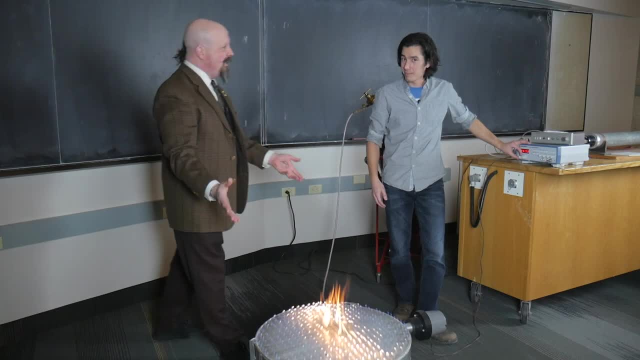 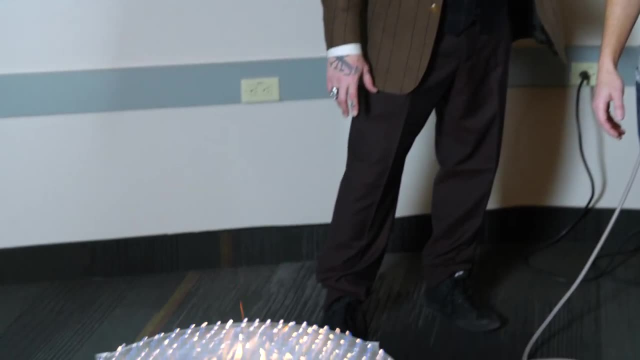 And you can see it now too, Again visually. we've got a 2D resonance taking place. You've got big pressure, low pressure, high fire, low fire. Okay, let's move it up to a higher frequency and see what else happens. 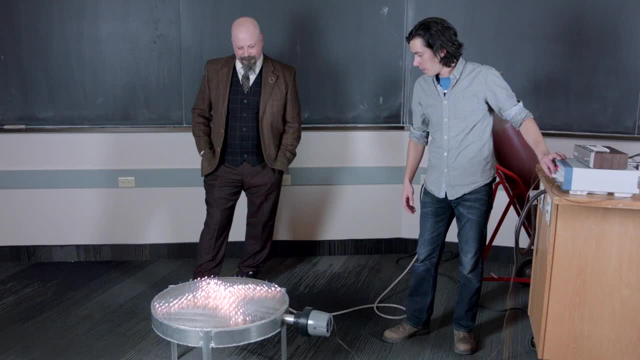 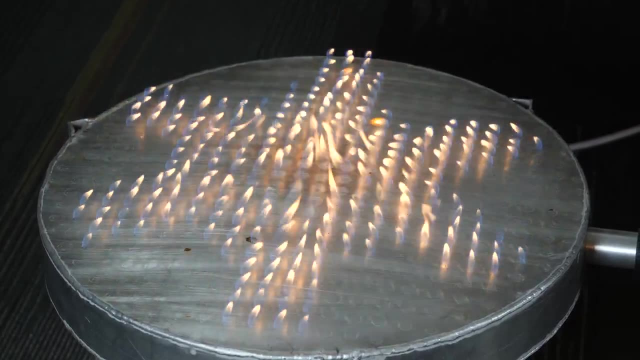 Oh, here we go. Okay, Let's keep bringing it up. So now we're gonna see three lines coming up next. But here you go. It's another visual interpretation of what resonance is. It's a bit more complex than the simple 1D example we saw before. 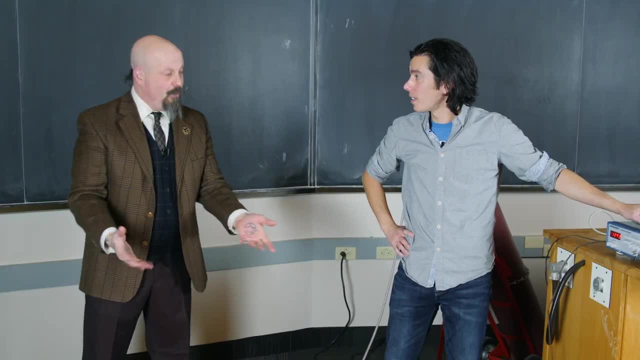 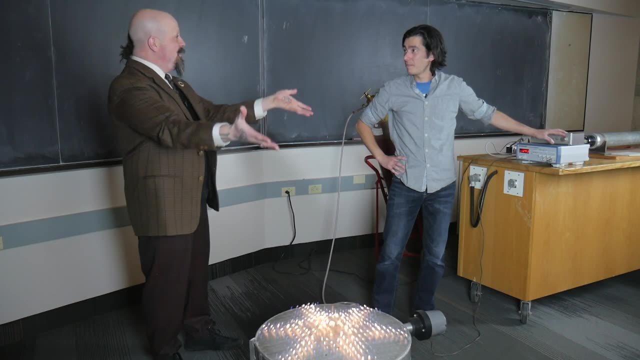 There's clearly more going on than just slapping in half wavelength intervals, but it's still resonance. You can hear it as the sound goes up and it increases in pitch. You can see it now as well, And so we have the definition of resonance here.